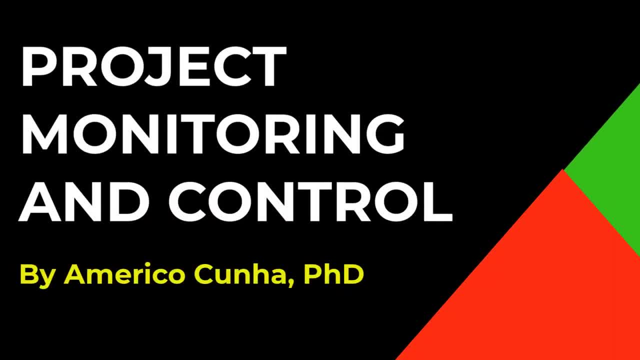 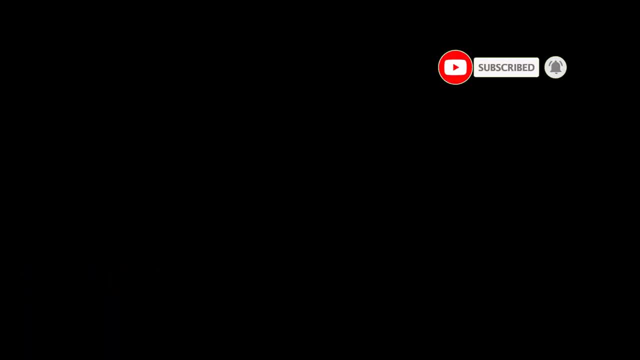 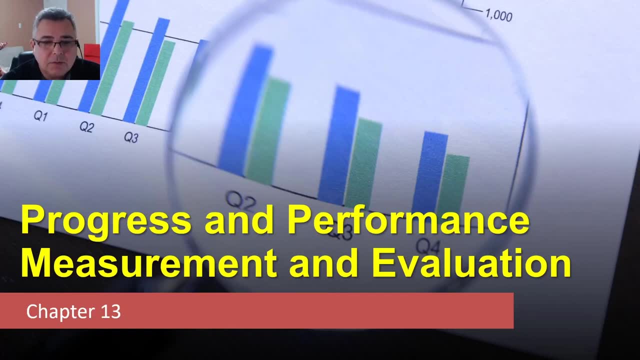 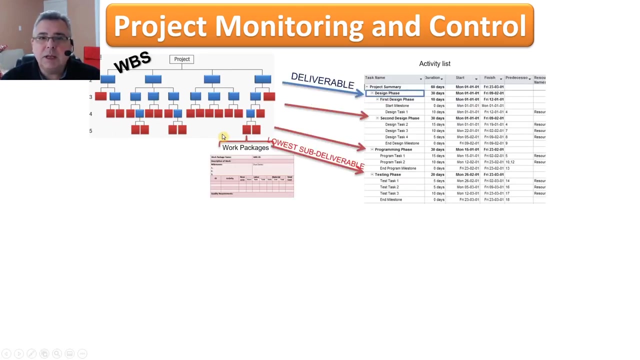 So today's class we are working on project progress and performance measurement and evaluation, That is Chapter 13, Larson and Gray book. and let's do it. So. we start with the scope, WBS, lowest level sub-deliverable work package. then we move those deliverables, sub-deliverables, activities to the MS project, prepare the activity list, estimate the duration, identify predecessors. then we move to the project network. then we elaborate the Gantt chart and then the time phase budget. 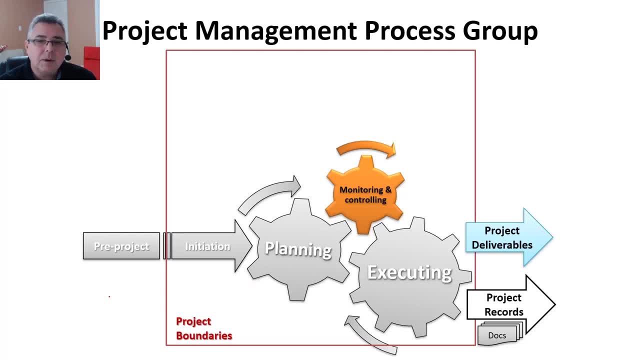 That is the planning process group according to the PMI. Today we are focused on monitoring and control, And let's dig a little bit deeper and understand what is monitor and control. Monitor and control have four major elements. Monitor is to observe. 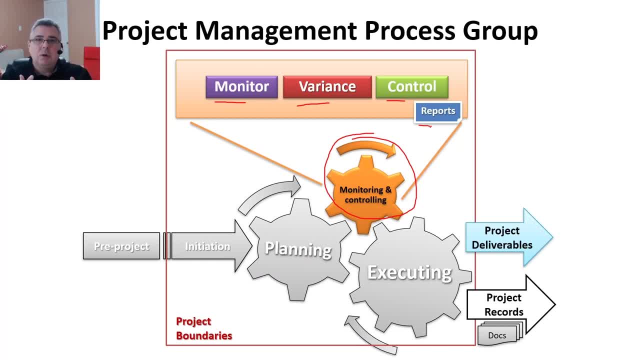 Observe. okay, When I call monitor, you are observing people doing the work. You are collecting information about the work done. okay, About the work. That's monitor. So one thing is collect information. The second thing is compare that information that is collected of the execution of the work done and compare that with the planning, with the project plan. 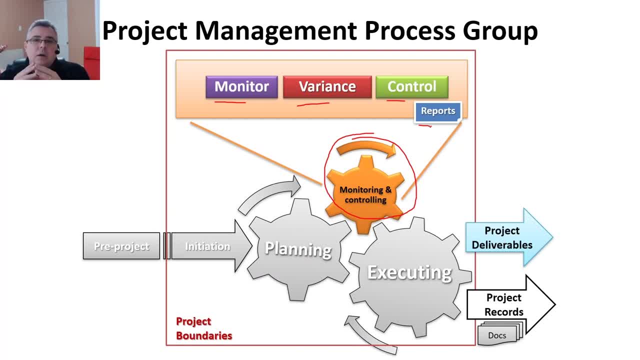 And here we are looking for variance. What is a variance? A variance is the difference between the work that was executed- Executed Minus Planning. Okay, That is what you call variance. If we don't have a variance, everything is okay. 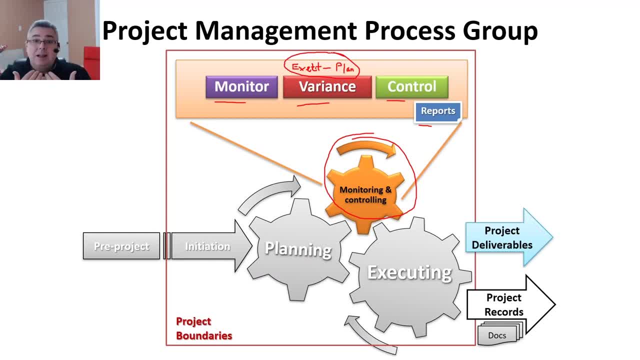 If we do have variance and depend on the level of variance, we need to act And that is the control. Sometimes you don't have to do anything or do nothing because everything is okay. Sometimes you have to correct things, Okay. 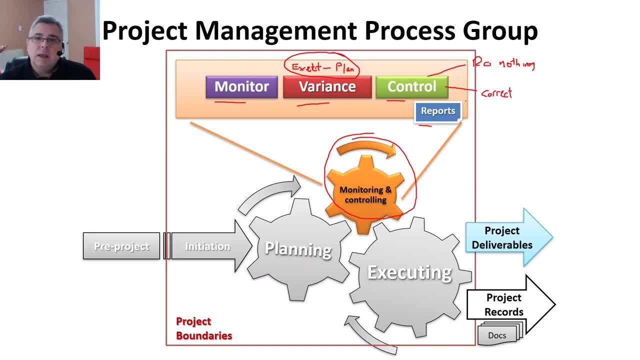 That is the function of controlling, And a critical moment for project managers during monitoring and control is to prepare reports, And there is one type of report that is called status report- Project status report that probably will have a huge influence in the project success. 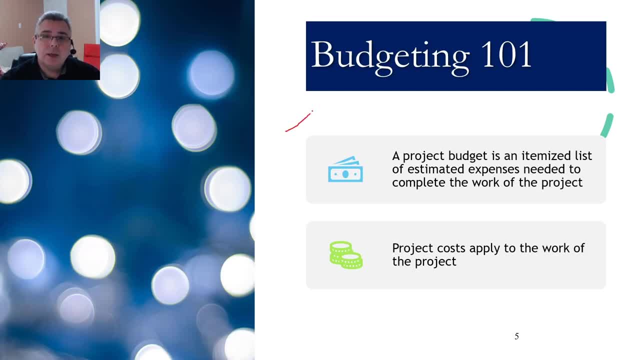 So during the project planning we have to do what The budget? The budget is an itemized list of estimated expenses needed to complete the work. And here we have two key points: Expense and the work. So we have in the budget: we attach expense to the work. 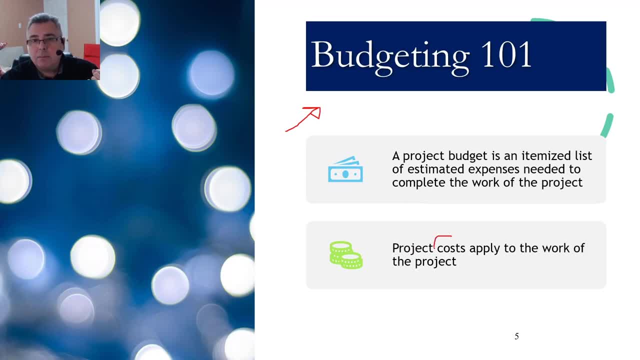 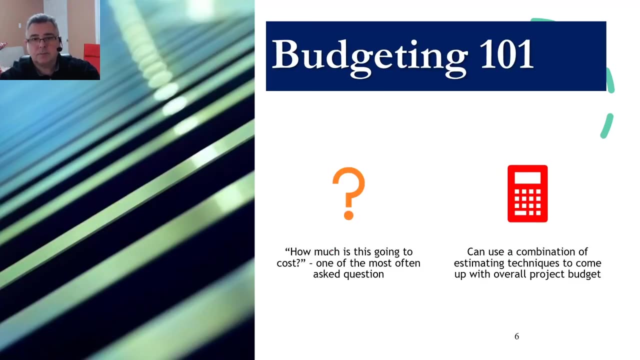 And that is important to understand. We have the plan costs, meaning the estimated costs and the work. That's very important to keep that in mind. So how much things the work is going to cost It's going to, That is future. 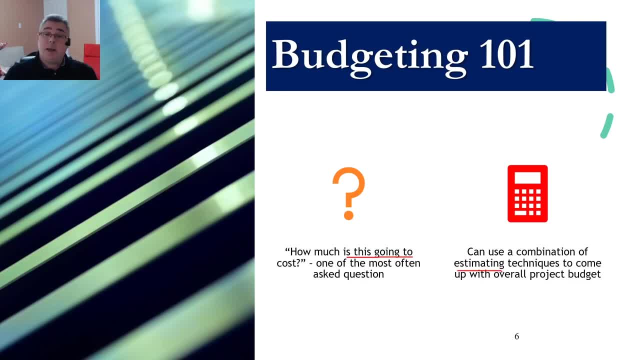 And this is estimate. It's not a real thing. It doesn't expect that the project will always follow the estimate. Probably not, And actually most of the time the project will not follow the estimate. Okay, But it's. 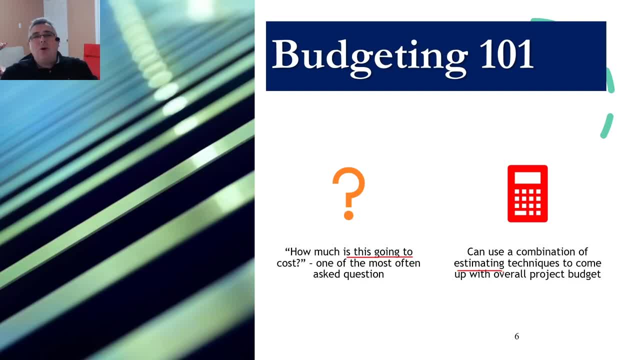 And there is a question that some people may ask me. So why do you need to plan for the project? Why? What do you think If I'm telling you that your estimates the reality will be different? So you need the goals and objectives. 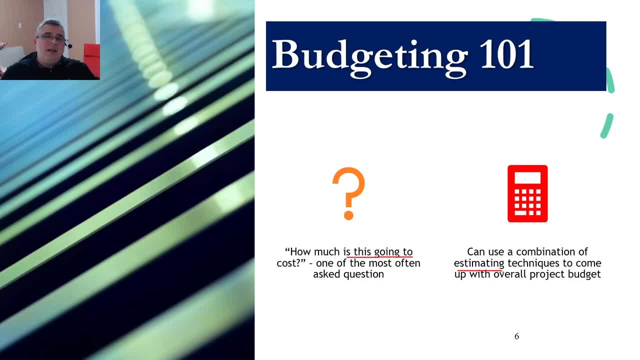 Yes, But mainly because you don't want to make a mistake of 600%. You want to Keep the mistake under 10%- 20%. That's why you need. So the estimate will be not exact, But at least you have a better direction. 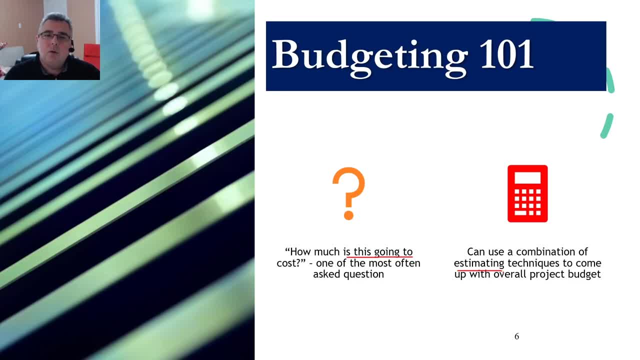 And the execution, if you do the plan well, will be close to the plan. It will be not. If you don't do any plan, you may have 600%. So you estimate $1,000 and go there And the real cost will be $10,000. 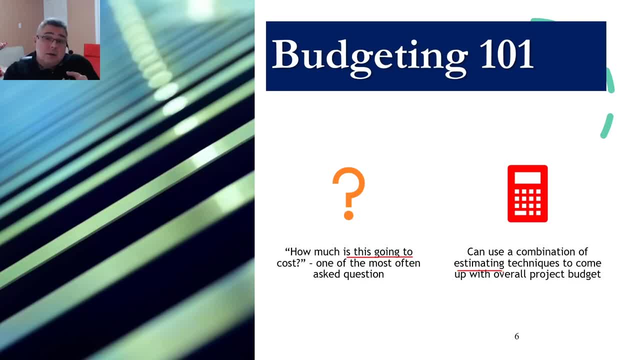 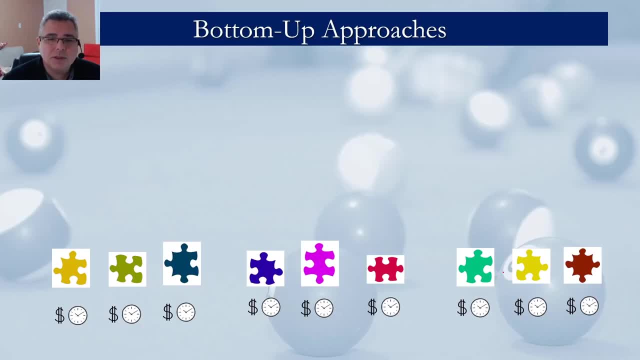 But if you do the plan, you plan $1,000.. But then the real cost will be $1,200.. $1,200.. Something like that. That's why we do this. Okay, We do the. 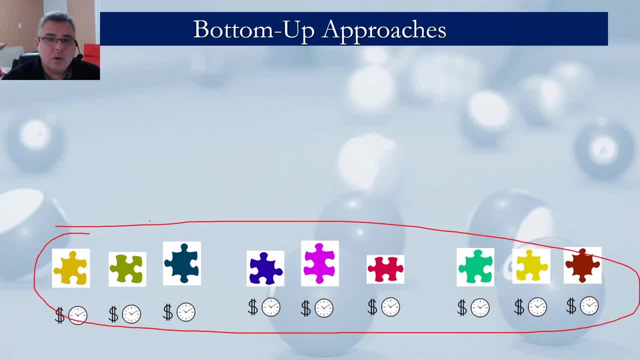 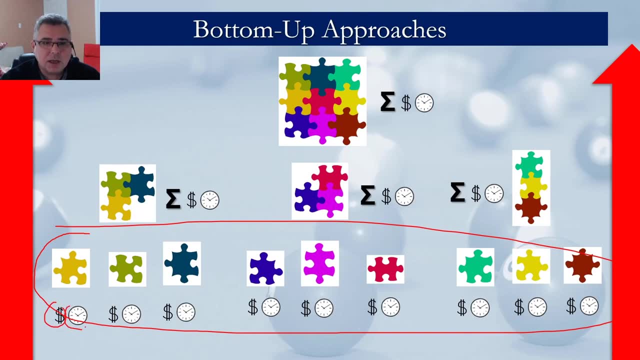 One of the ways of doing that is doing the borrow-wap approach, parametric approach. We studied that at the beginning of Chapter 5.. So you go from the cost and duration of each task lowest level deliverable, the work package. 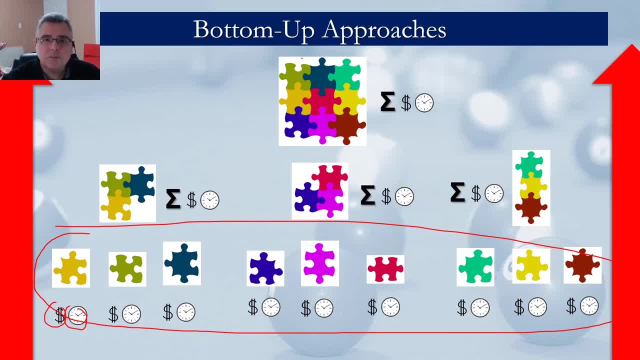 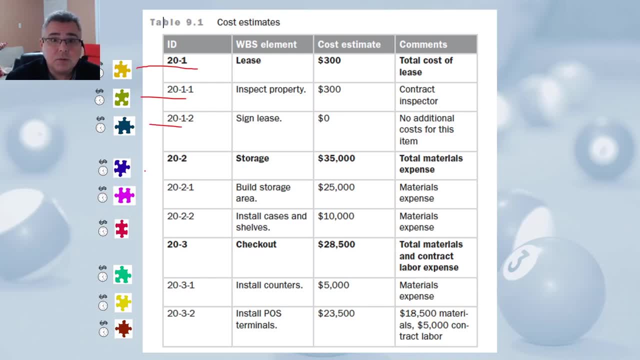 is going up until you have the cost and time for the whole project. That is what you do, How that Reflects on the budget. So you have each task of the lowest level sub-deliverable. You have to understand that task and the cost for each task. 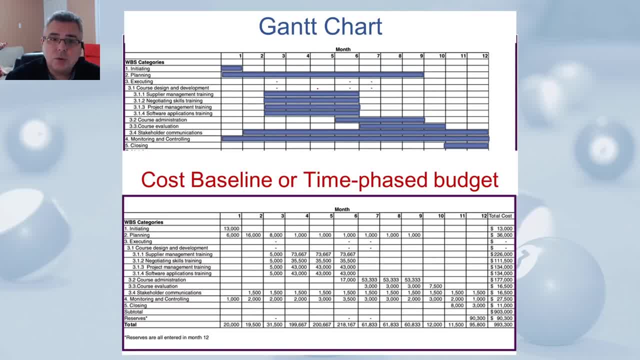 So that is the budget, And after doing that, we need to place the expense throughout the project time frame. So and we go for: You have the gun chart from the scheduling plan And you have the time phase budget, And so we just put the expense. 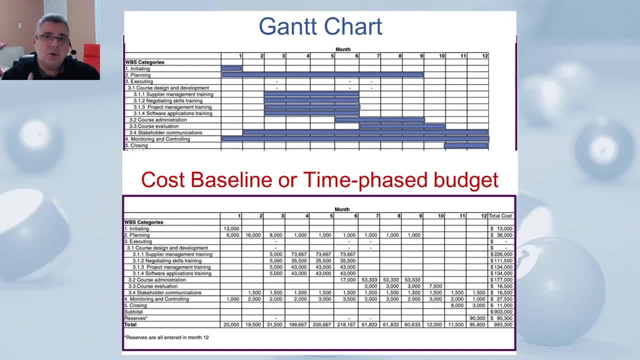 So the expense relate to activity during the time you are executing the activity. So if you have one activity here, that's the expense for that activity And that will be when you are expecting the project manager is expecting to incur on. 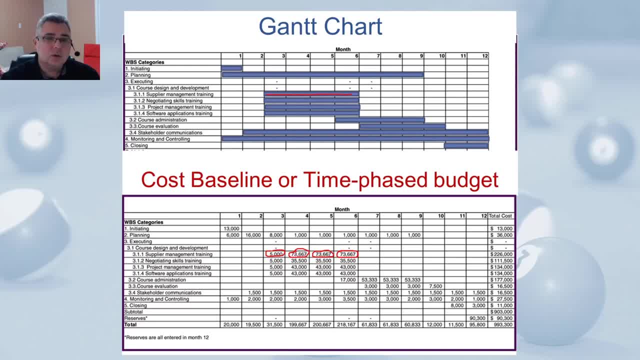 those expense, Pay those bills. Okay, Use that money. So that's very important when you do the planning. So everything here Represents two things: The time and the money. So that's why cost baseline or time phase budget are so critical in the project planning. 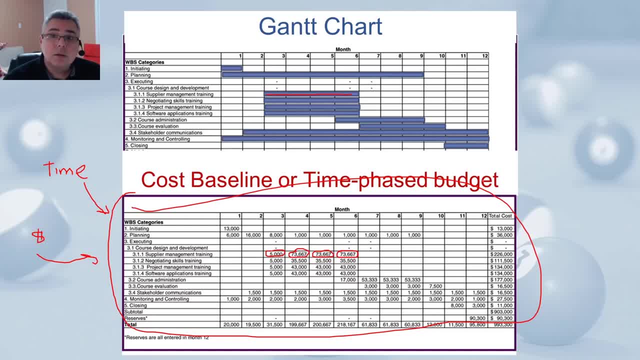 Because that time phase budget consolidates the time from the gun chart, from scheduling, plus the budget Put two things together. That's simple. That's simple. That's a simple table. Okay, That's very important. So everything that we do and that cost baseline is or time phase, but it's the main. 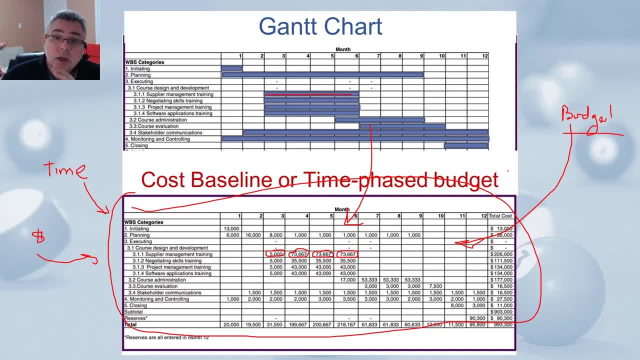 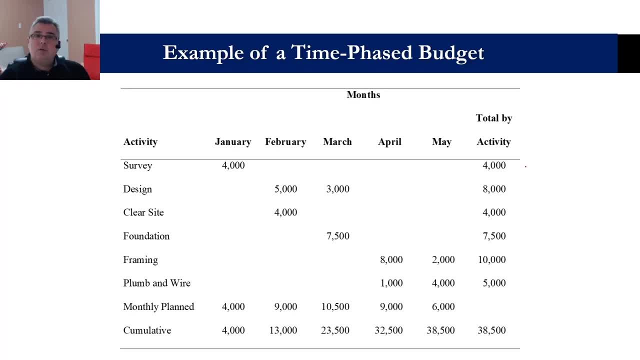 resource or input for monitoring and controlling the project. Okay, Because it consolidates time and the budget. So that's a beautiful time phase budget And everything that we'll be doing here in terms of monitoring and controlling. we'll be collecting information from the time phase budget. 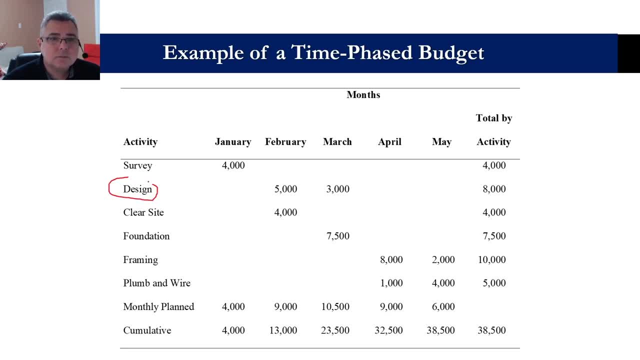 Because here let's take the one activity here: design. You know that design will be executed February, March and you have $5,000 of expenses In February, $3,000 in March. So you know that there is amount of work that should be done in February. 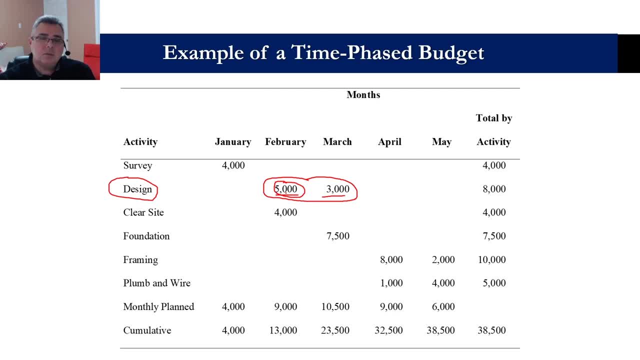 Okay, In February of $5,000,, like I said, you have $5,000 of work to be done in February. In March, you have $3,000 of work to be executed in March. Okay, So time phase budget is the main input for project monitoring and control. 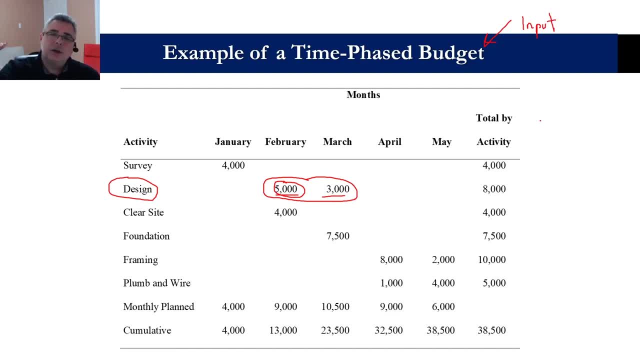 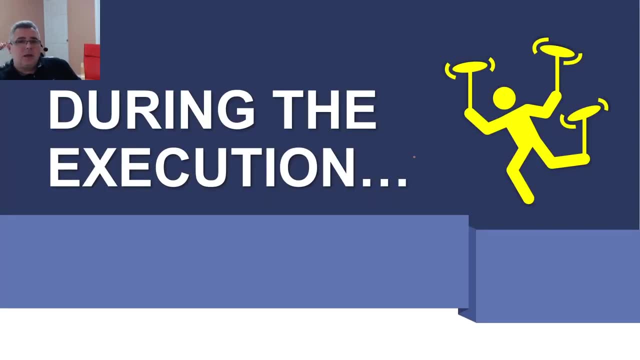 Of course, because if you think about gun chart is here, the budget is here, project budget is here. So that is the main report that you may use for the project control product or the project. Okay, When you finish the plan after the time phase budget, you finish the plan, maybe two. 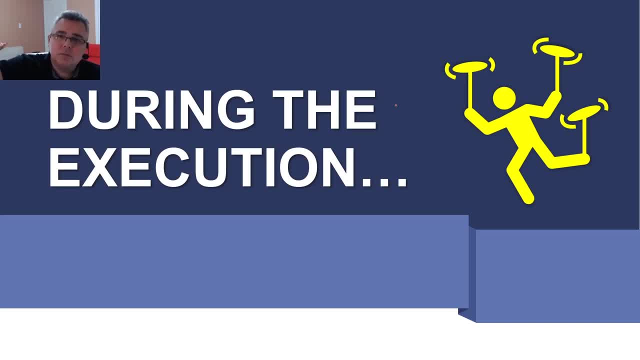 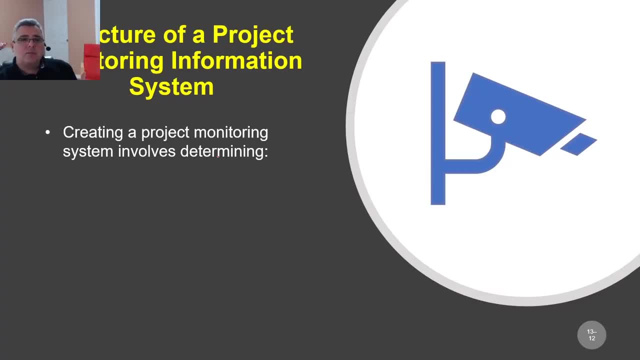 weeks later, one month later, you start the execution, You start doing the execution And, now that you have the plan, when you start the execution you have to create a system that allows you to collect data, Because, as a project manager, you don't know what's happening in the field. 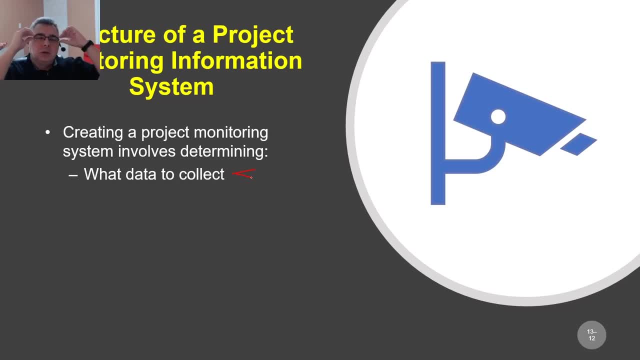 In some projects you can, You can observe, But in big projects your contact with the person that is executing the task is very low. You don't see it. Sometimes it's in another city, in another province, It's not the same. 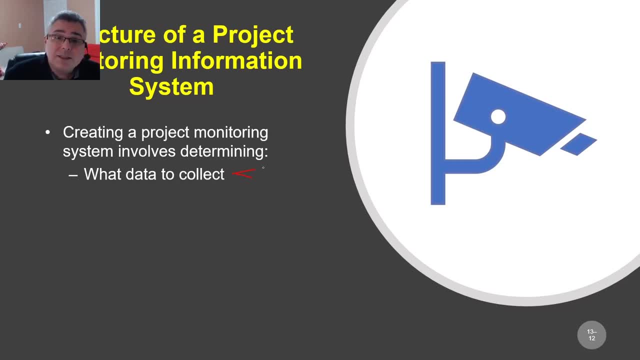 So you have to collect that data from the execution. What is the data from the execution? Time spent, Okay, Time spent on the task. You need to know how the time spent on the task. You, as a project manager, know the plan. 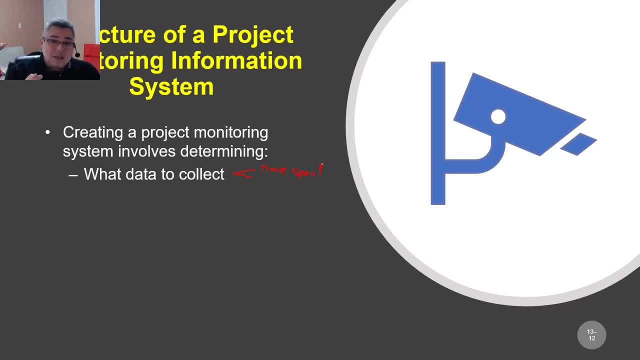 You know what is the estimate, what you are expecting, But you need to get- and you just know that if you contact the person that is in charge for the task- Okay. Another thing is the actual cost. You estimate, like I said, that design activity, in that work, in that project, the estimated. 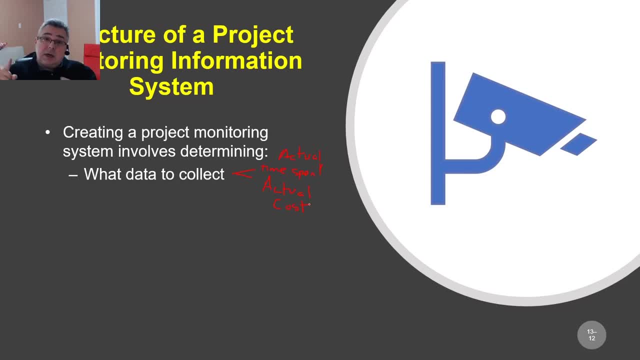 cost $5,000.. But when they start, the person that is in charge starts spending money. you don't know if the person has spent $5,000 or the same thing. you estimate: maybe the person has spent $6,000, maybe $4,000. 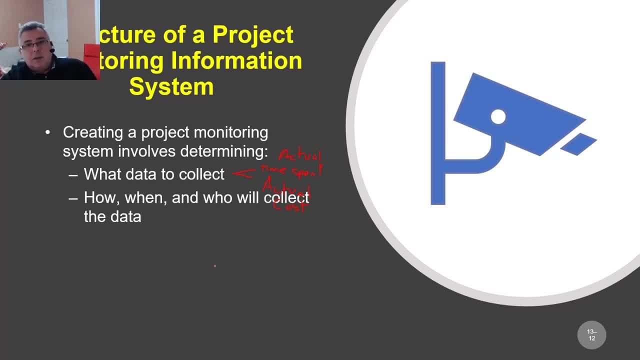 You don't know. You have to collect that data. And to collect the data, Of course, you have to collect the data. You have to collect the data, You have to collect the data. Of course, the major, major element is to know who is the person. 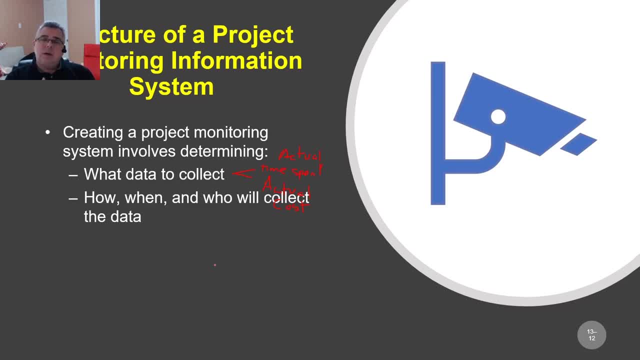 And that's why you need to have a good race, at least a good list of project team with emails, telephone numbers, contact information and know who is the executor and who is the manager for that executor accountable person. It's important because if the guy doesn't answer your questions, you go to the manager. 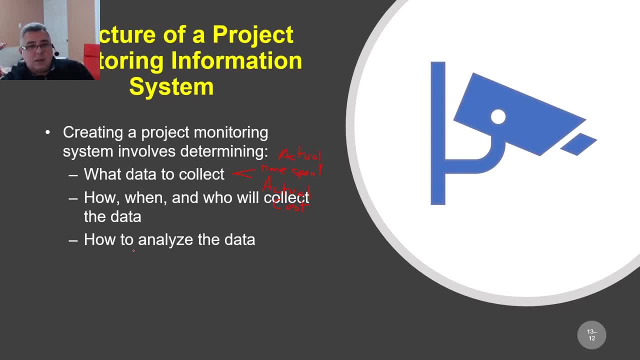 Okay, So that's important to understand- and how you'll be analyzing that data that you collect from the field. You'll be comparing that with the information that you have on the time phase budget. Okay, Time phase budget. That is the main, main thing that we need to understand. 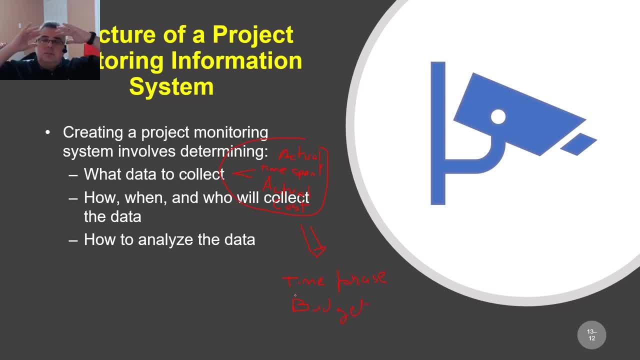 So we are now with your mind. You have to Okay, So, Okay. So we are now with your mind. You have to somehow forget your planning activities. You are not planning the project anymore, So most of the things that you have done so far in the planning was done maybe two weeks. 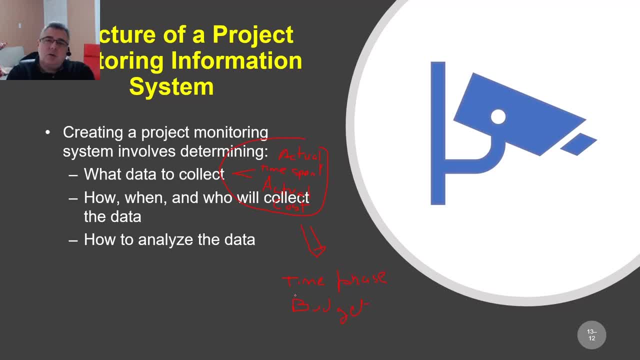 ago, one month ago, and now you are in the middle of the execution And that is the job I would say that you'll be doing routinely, every day in your life, Because 80% of the time you'll be contacting people, understand, collecting data. 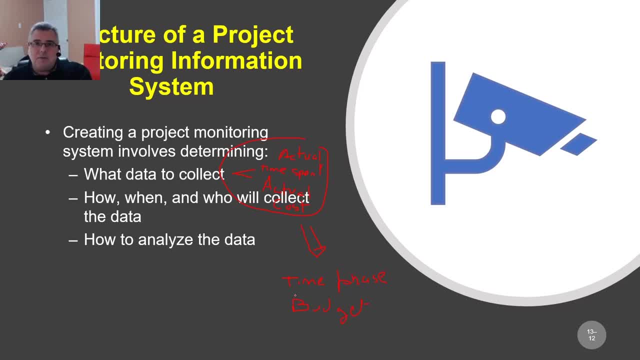 Okay, and that is every day: prepare your time, phase budget, take some conclusion, discuss some, some actions to correct the project. so that is the job that you'll be doing 80 of the time. everything that you are studying in this semester is just 20 of your time as a project. planning should be less. 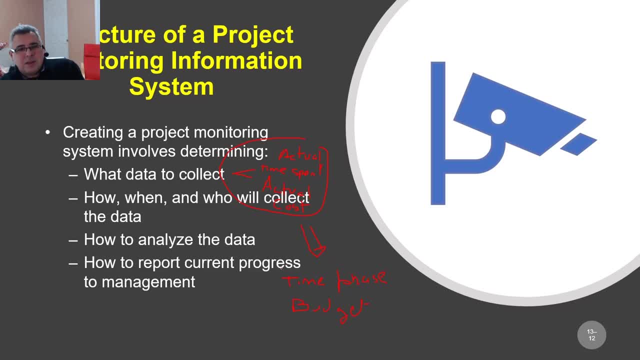 than 20 actually, if possible, and that is a critical thing if you want to get your project have success: how to report the progress, because how the project manager report the project, that guide the team, that influence the decision makers, like managers and executives, it so how you be reporting the information from the project will help you to solve things or not. 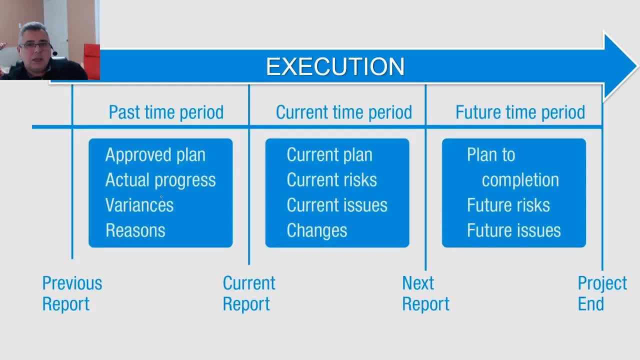 okay, that's very, very, very important. so let's, let's see what i am explaining in a in a different perspective. that is the current report. you are here to take that as a timeline. so you have been a shopping center, is that that you are here, okay? 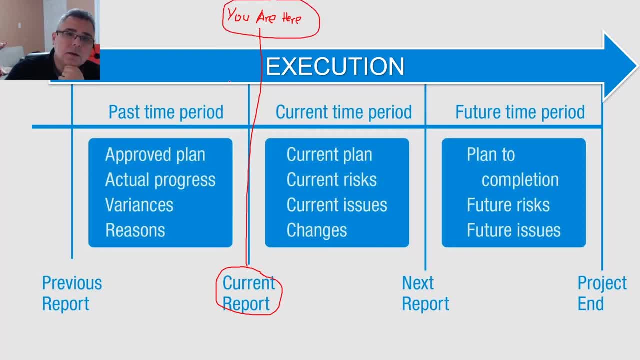 you are here and what's happened? you have done the planning some time ago. okay, you have done the planning maybe two months ago, four weeks ago, five weeks ago, and now you are executing. so then your project is going week by week, month by month. so if you are here, you look, have to look back and you have to collect information. 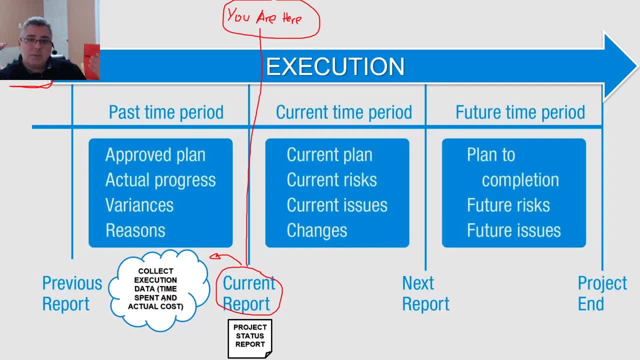 from collect execution data, time spent and actual cost, because you have to collect- and this you have to contact the executor, the managers, uh, if you have to call or ask them send their emails or meetings, whatever, but you have to collect those information. and what do you do with that information? 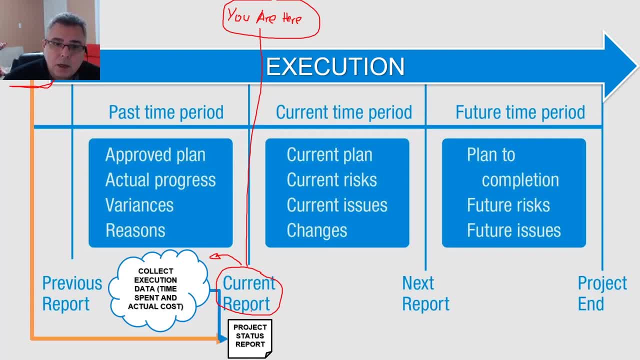 you compare with the planning and you issue a status report. project status report: that is the main thing that you have to do. okay, issue that project and that project start report will be talking about the consequences of the variance here. moving forward, if someone is late, you have to. what is the consequence of that task that is late? 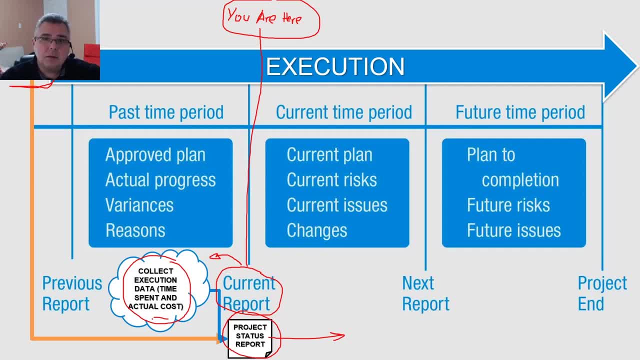 if someone spent more money than the budget, what are the consequences for the project? so, as a, as a project manager, one job that you have to do every week, and that is is to issue a status report every week. every week in your life as project manager, you have to issue a status report. okay, and usually that that's why 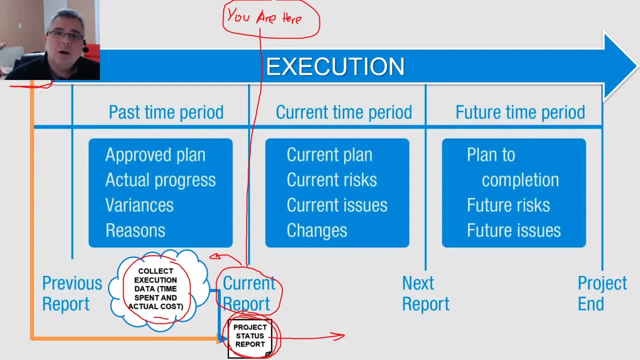 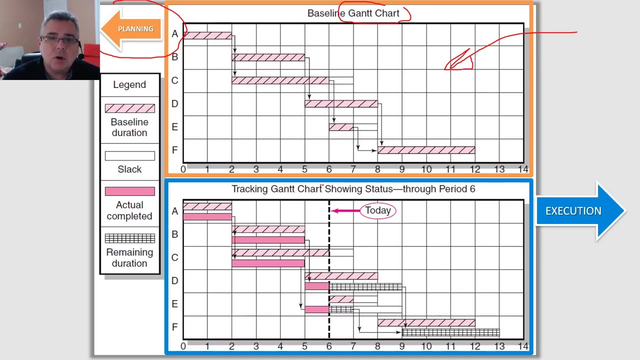 you, you'll be spent most of the time again, around 80 percent or more of your time, 80 percent or more of your time here doing that, that type of work. for simple projects, you can track the performance using what is called tracking gun chart. actually, even for you can. 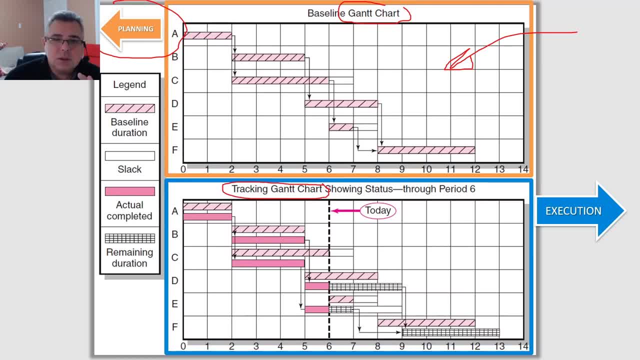 get that from ms project as well. but this you, you have just, uh, you can visualize the work execution. you don't have information. you don't have information about the work execution. you don't have information about the work execution. you don't have information about costs, just about the execution. so let's suppose 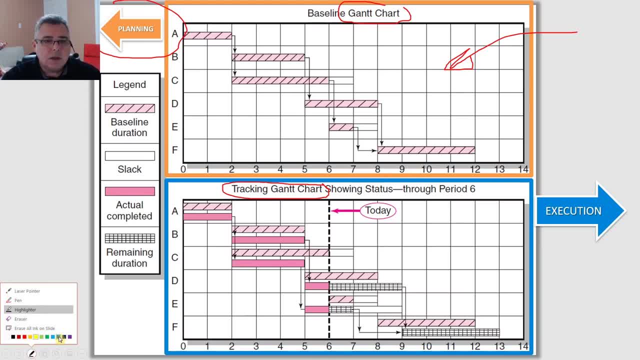 costs just about the execution. so let's suppose costs just about the execution. so let's suppose that you have uh, that, you have uh, that you have uh here, let's put in here, let's put in here, let's put in. was the planning? okay, that was the. 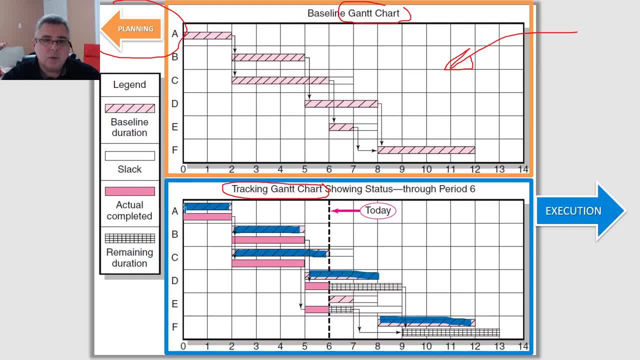 was the planning? okay, that was the. was the planning? okay, that was the planning, planning, planning. so that's the way you you plan task a, b, c. so that's the way you you plan task a, b, c. so that's the way you you plan task a, b, c, and in red is the execution. it means that task. 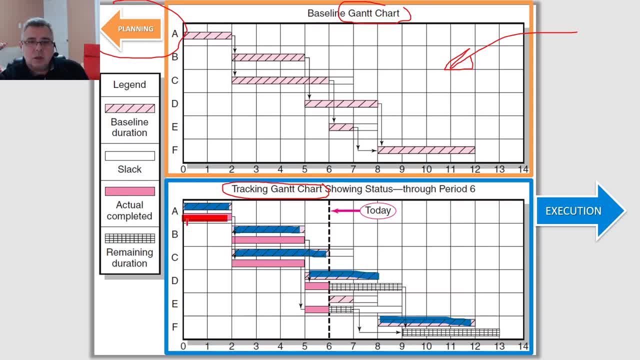 and in red is the execution, it means that task and in red is the execution, it means that task. a was planned to be executed up to day two. a was planned to be executed up to day two. a was planned to be executed up to day two and it was executed. the blue means the. 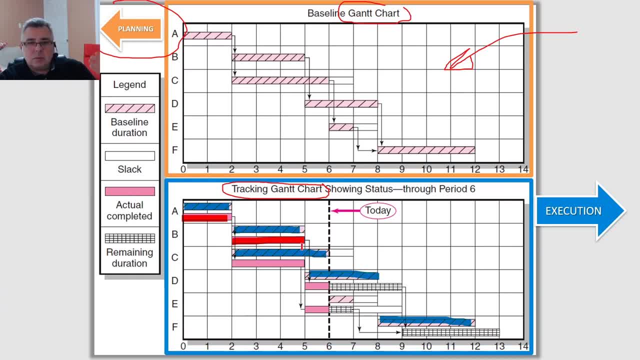 and it was executed. the blue means the and it was executed. the blue means the execution, execution, execution. task c. it means that, should you plan to task c. it means that, should you plan to task c, it means that, should you plan to execute the tasks b- sorry b- from day two. 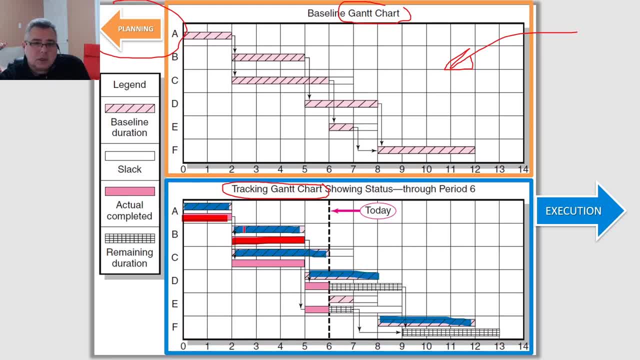 execute the tasks b, sorry b, from day two. execute the tasks b, sorry b, from day two to day five, to day five, to day five, and, and. and. you execute the task. you execute the task. you execute the task. task c is different. can you see task c? 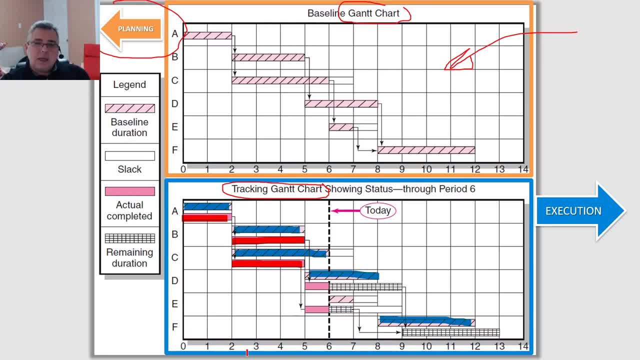 task c is different. can you see task c? task c is different. can you see task c? what's happened to task c? it took less. what's happened to task c? it took less. what's happened to task c? it took less time than expected? yes, exactly because 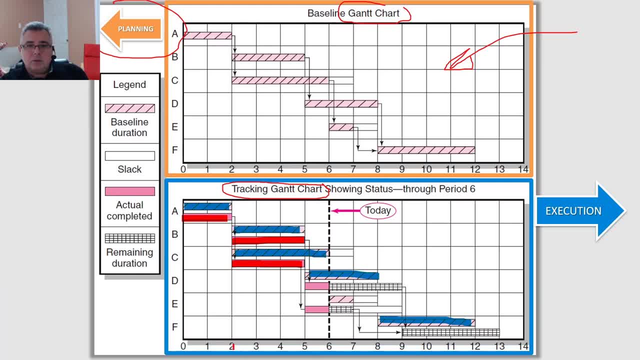 time than expected. yes, exactly because time than expected. yes, exactly because you was ex during the planning. you saw you was ex during the planning. you saw you was ex during the planning. you saw that you would be from day that you would be from day that. you would be from day two. 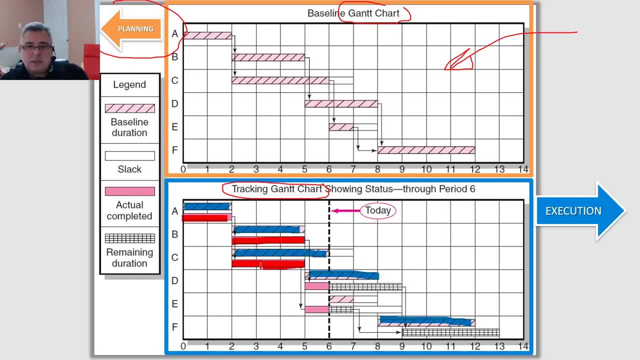 two. two to day six, but to day six, but to day six. but for some reason, the guys there, for some reason, the guys there, for some reason, the guys there execute the task, execute the task. execute the task in three days instead of four, now you. in three days instead of four, now you. 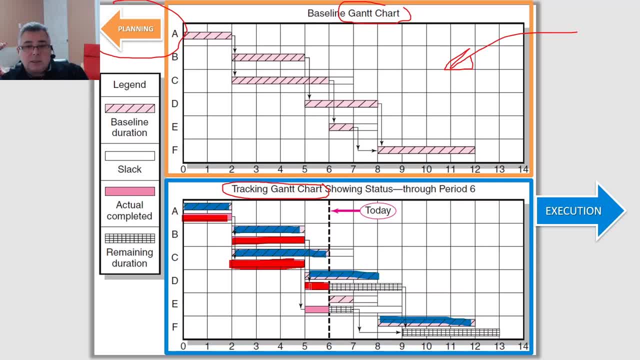 in three days instead of four. now you have. if you are here, that's today. have if you are here, that's today. have if you are here, that's today. what's happened to task d? how can i what's happened to task d? how can i what's happened to task d? how can i interpret that situation of task d? it? 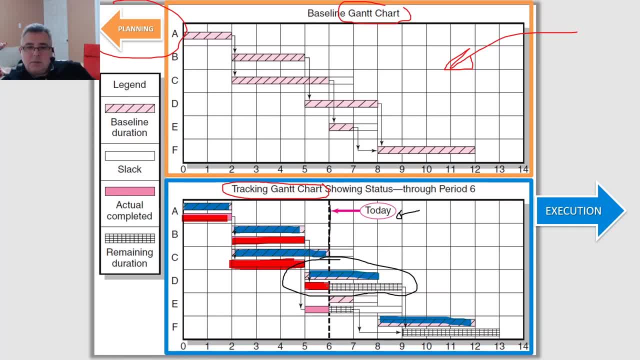 interpret that situation of task d it. interpret that situation of task d it started you. you plan to execute in, started you. you plan to execute in, started you. you plan to execute in three days. somehow, three days, somehow, three days, somehow. you are, you are, you are. after the first day you come back and talk. 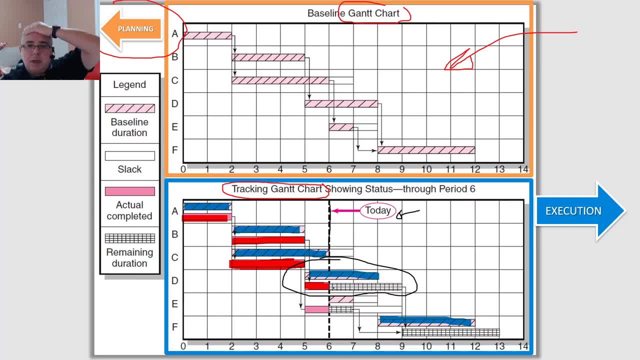 after the first day you come back and talk. after the first day, you come back and talk to the person in charge for the task, to the person in charge for the task, to the person in charge for the task, and that person maybe has told you that, and that person maybe has told you that. 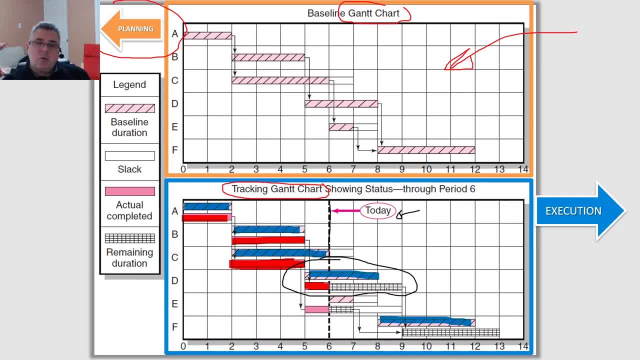 and that person maybe has told you that he's late and you may one thing that we he's late and you may one thing that we he's late and you may one thing that we always ask is: what have you done? always ask is what have you done? 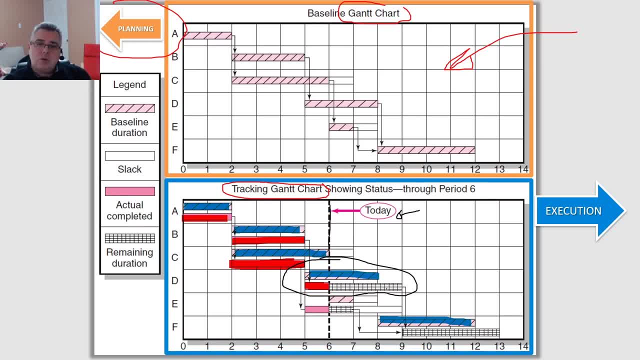 always ask is: what have you done? and the second question has always been, and the second question has always been, and the second question has always been: how long do you think it will take to? how long do you think it will take to? how long do you think it will take to complete the task? and probably the 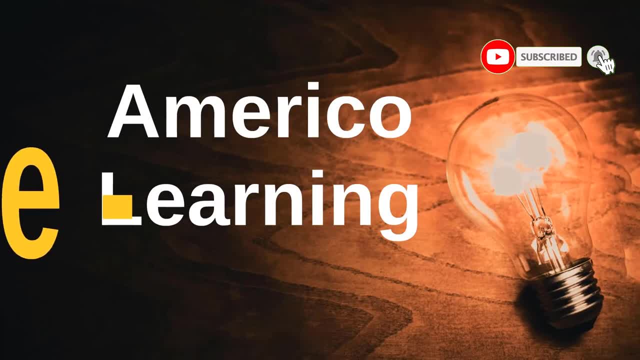 complete the task and probably the complete the task and probably the person told you three days person told you three days. person told you three days. we worked hard to help you to get better. we worked hard to help you to get better. we worked hard to help you to get better marks. 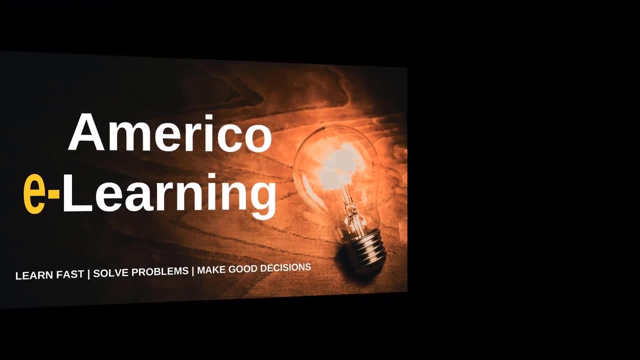 marks marks prepared for job interviews and excel in prepared for job interviews and excel in prepared for job interviews and excel in work meetings- work meetings, work meetings. you can send your questions in the. you can send your questions in the. you can send your questions in the comment area below. 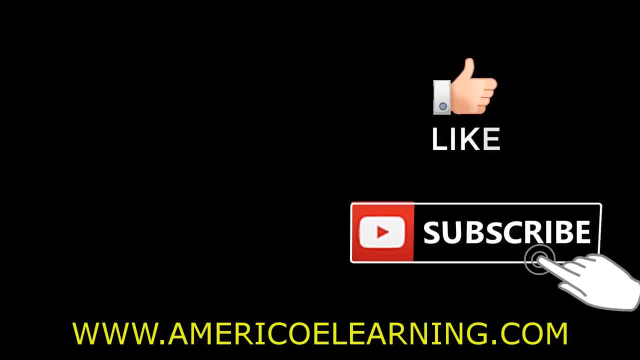 comment area below. comment area below. i will be pleased to answer all of them. i will be pleased to answer all of them. i will be pleased to answer all of them. thanks for watching. thanks for watching. Don't forget to subscribe to Américo e-Learning.